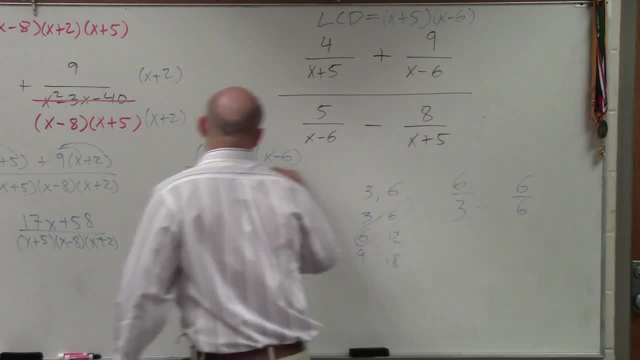 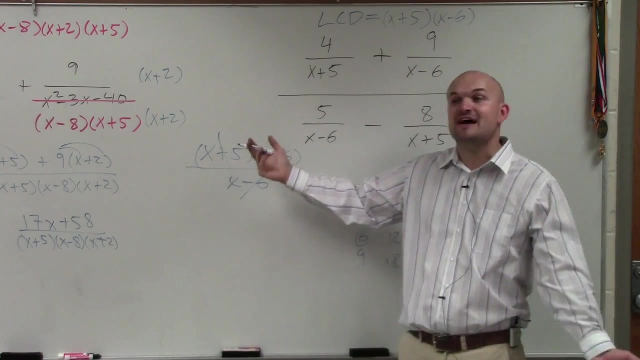 So you take your common denominator and you say: hey, does X plus 5 divide into that? Sure, it does X minus 6 times, right. And then you say: does X minus 6 divide into that? Sure, it does right, Because that divides the 1. It goes in there: X plus 5 times. 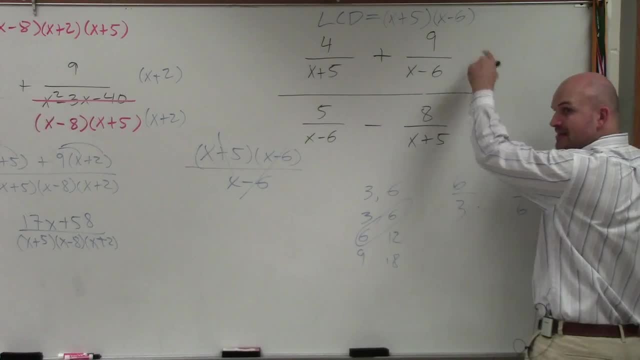 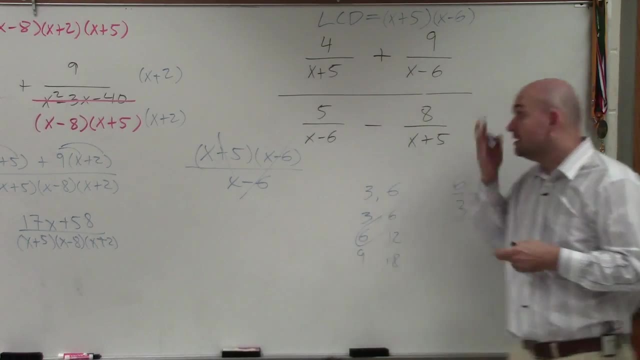 So do you now agree with me that all of these divide into that common denominator? That's why just multiplying the denominator is so helpful when you have polynomials, because it's always going to produce you something they divide into. So now I'm going to multiply everything by my LCD. 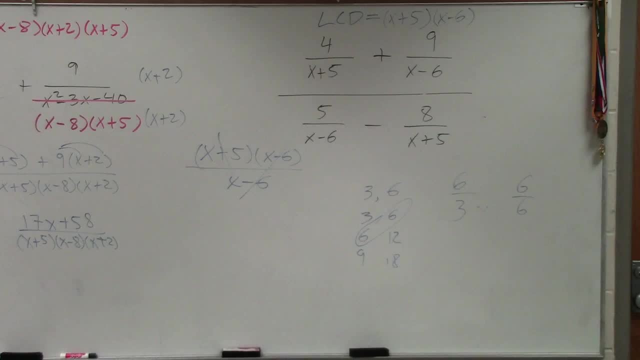 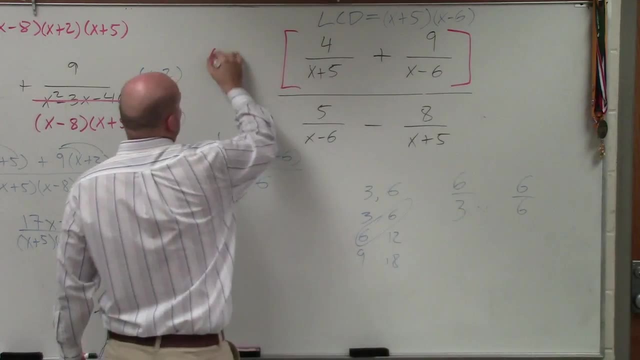 No, no, you need me to help you. Oh sorry, Trash can's over there. I know it's sometimes hard to get over there. So you have to multiply your numerator and your denominator. So you have to multiply your numerator and denominator by your LCD. 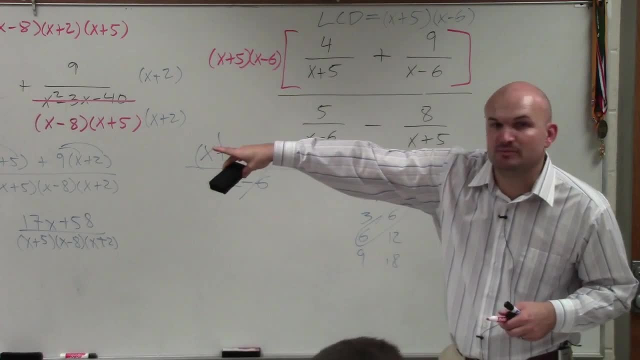 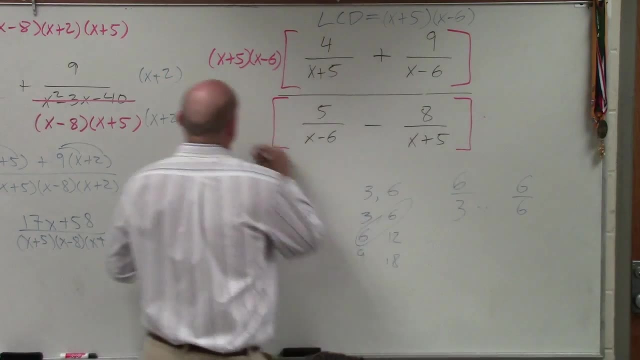 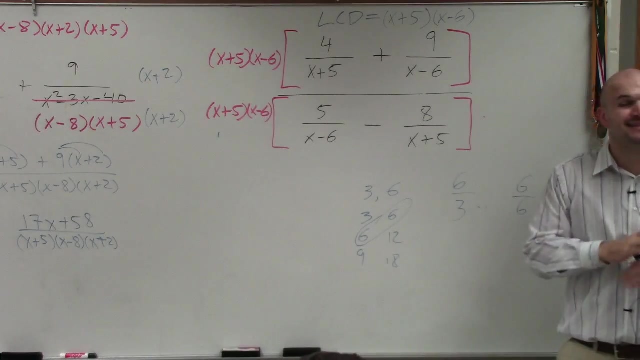 Remember? see how I multiplied the numerator and denominator. I'm going to do the same thing over here, but my goal in this case is not to produce equivalent denominators. My goal this time is to eliminate the denominators. Now notice how this is an expression. This would be like X plus 4 or something. 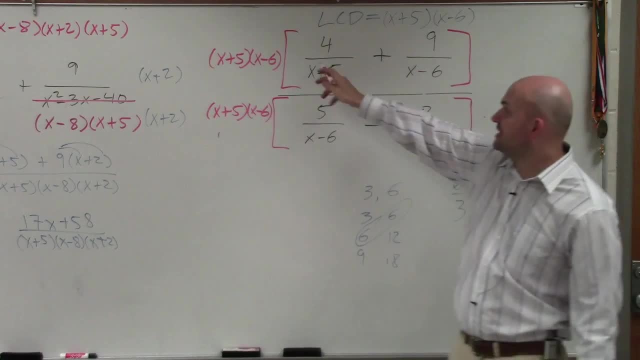 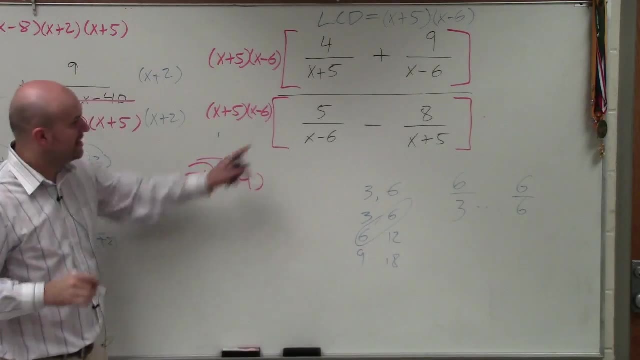 You have to multiply times both of them, Right? You can't see how these are separated: 5 times X plus 4.. You have to apply distributive property, Right? These fractions are separated by addition and subtraction. You have to apply distributive property. 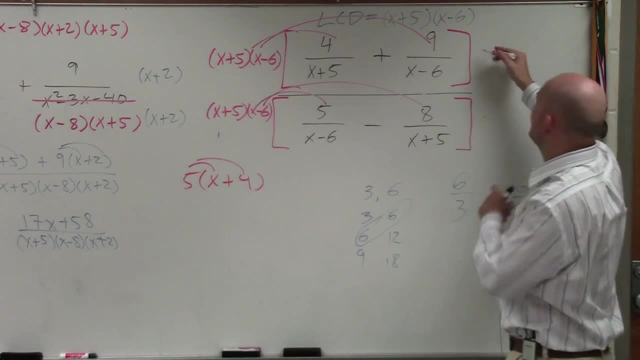 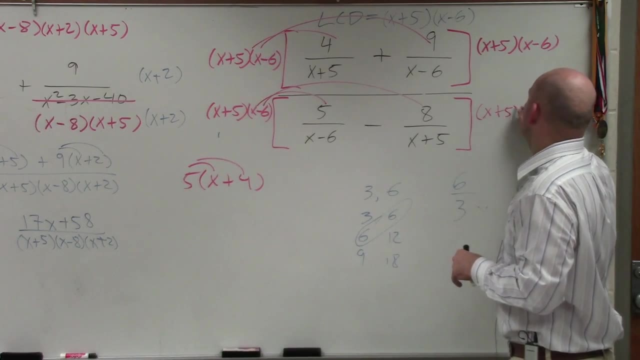 Yes, Right, So in reality I'm just going to write it over here to make it more sense. So I'm going to say: the product of this times, that and this times that. Now let's have fun. Let's have fun using the zero product property. 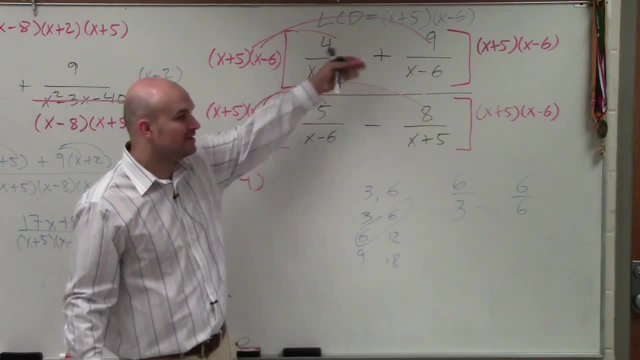 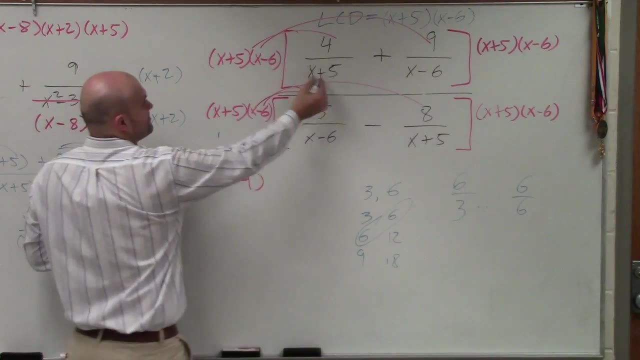 Once you understand, you take for complex fractions. when you have an expression divided by another expression with fractions, multiply everything by LCD. Let's see what happens. Well, here X plus 5 divides into it. Right Here, X plus 6 divides into it.